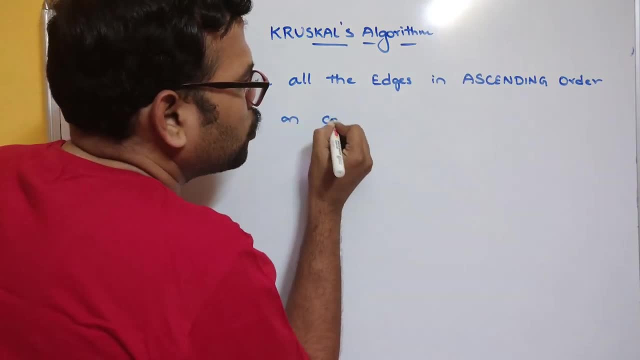 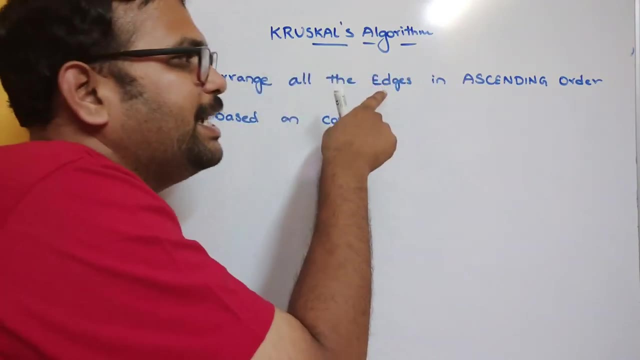 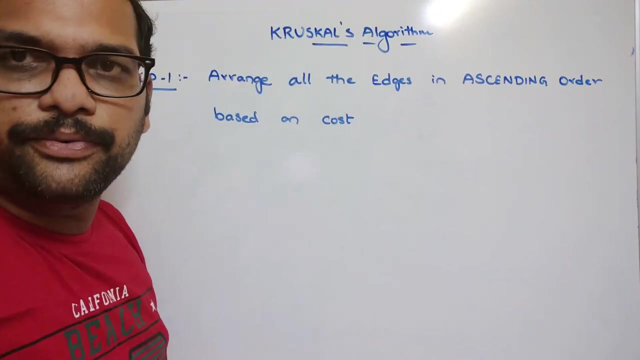 each of this ascending order based on cost. so every edge will be having their own cost. so we need to first arrange all the edges in ascending order based upon the cost right ascending order means lower value to the higher value, so we need to find the minimum cost spanning. 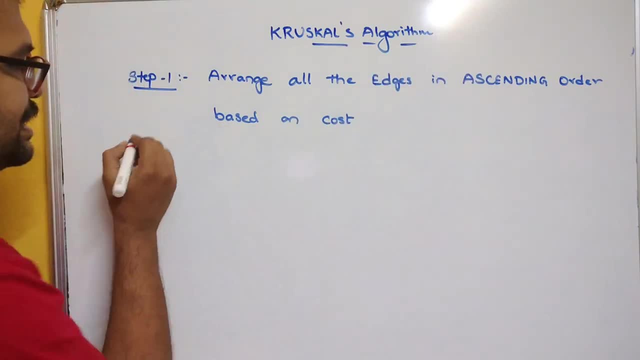 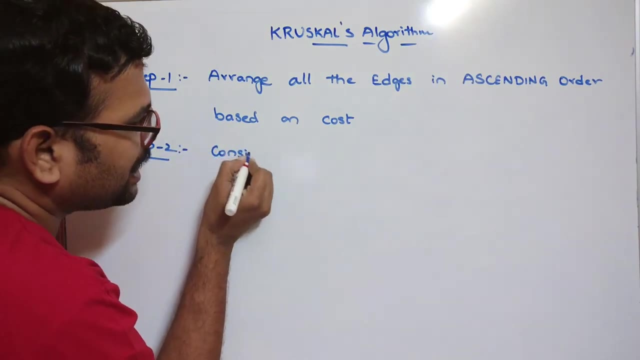 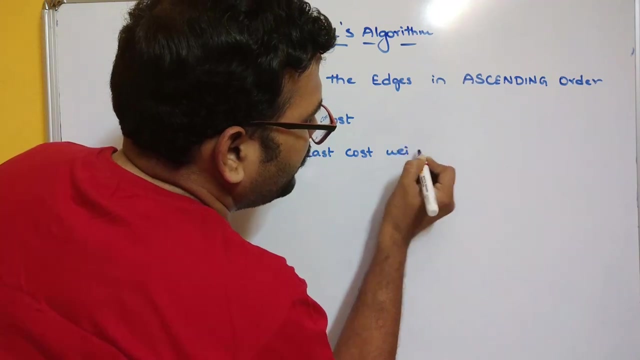 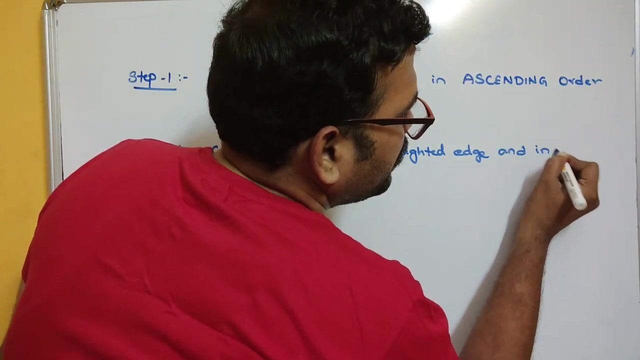 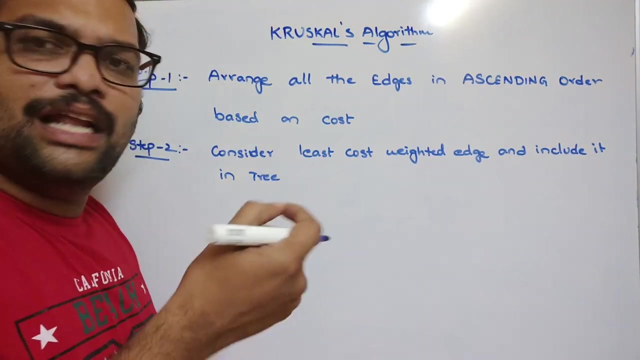 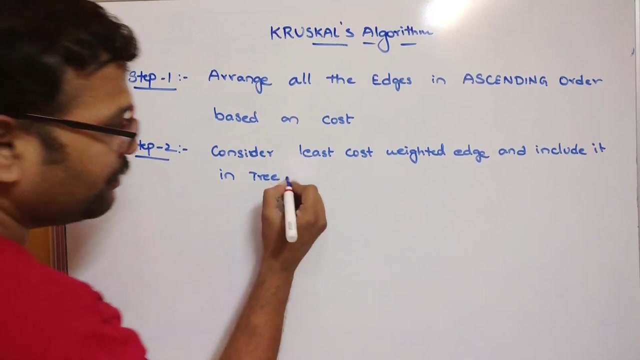 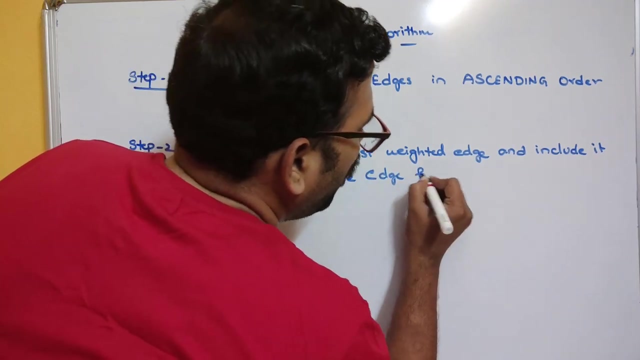 tree. so that's why we are using this ascending order. and the next step 2, step 2: consider, consider least cost weighted edge and include in the tree. Include it in tree. So consider one by one and just include that in a tree And if, if the edge forms a cycle, forms a cycle. 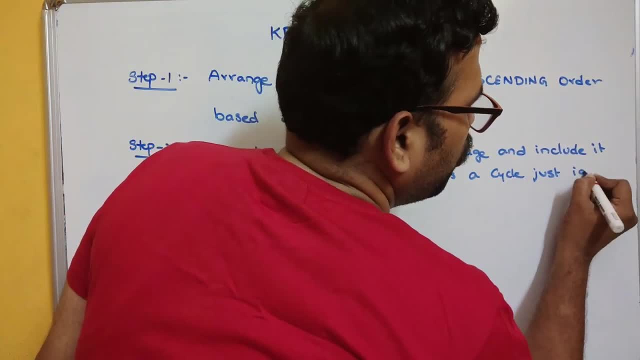 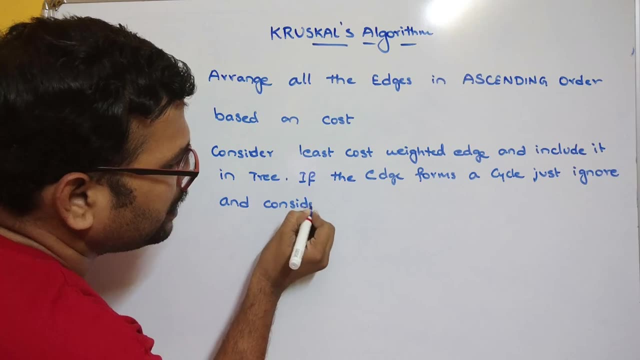 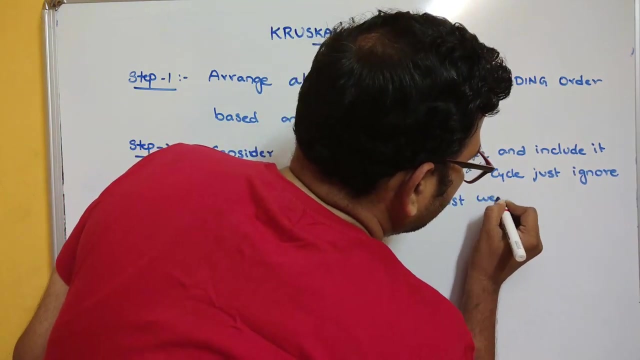 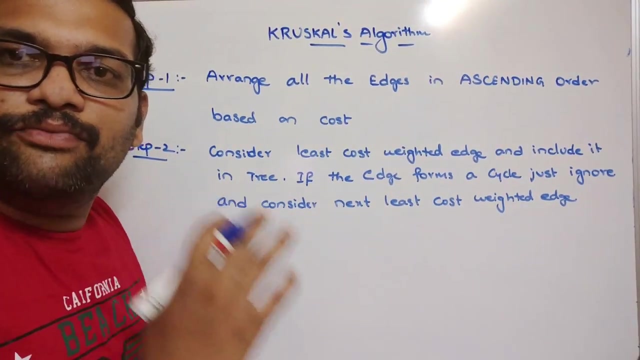 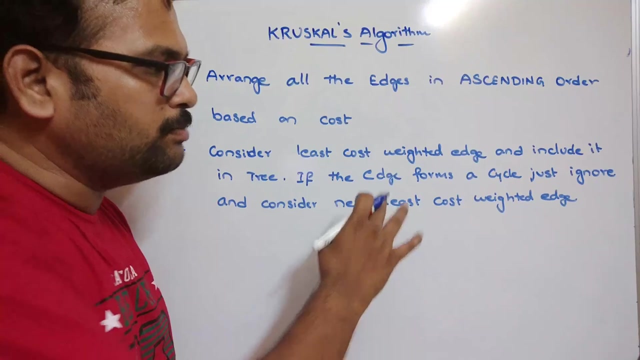 just ignore and consider. consider next: least cost weighted edge, least cost weighted edge. So every time we'll consider an edge and we have to include that on a tree. So if, if, by adding that edge, if it forms any cycle, so just we have. 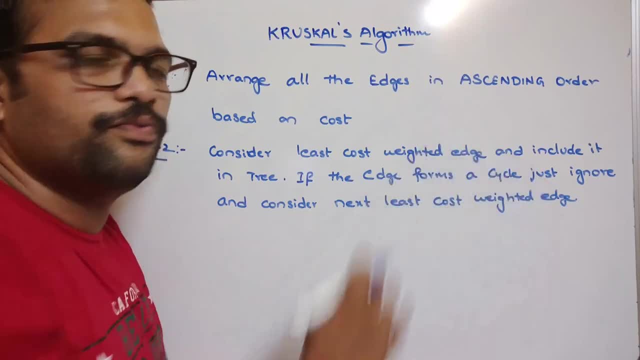 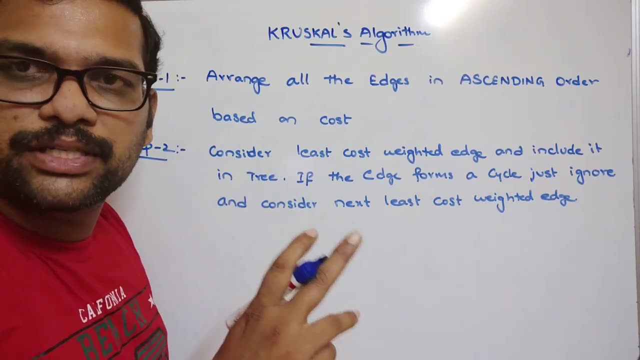 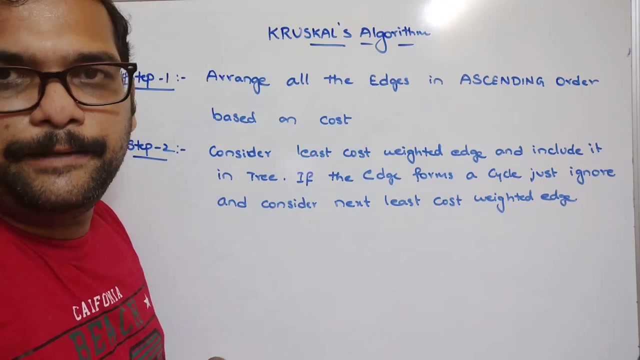 to ignore that edge and consider the next least cost weighted edge, because a tree should not have the cycles right. So graph can have the cycles, but the tree should not have the cycles. So here we are, using this Kruskal's algorithm to find the minimum cost spanning tree right. 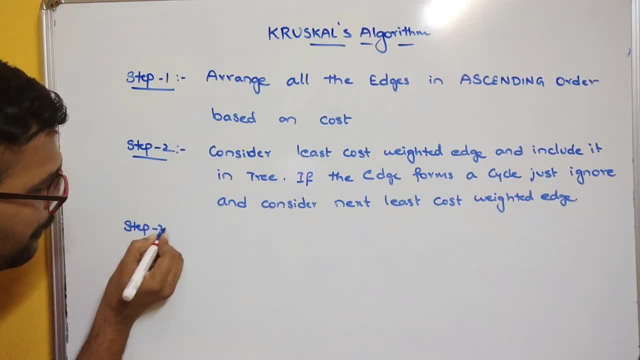 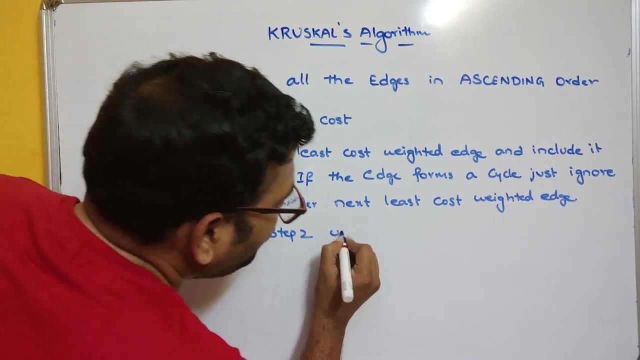 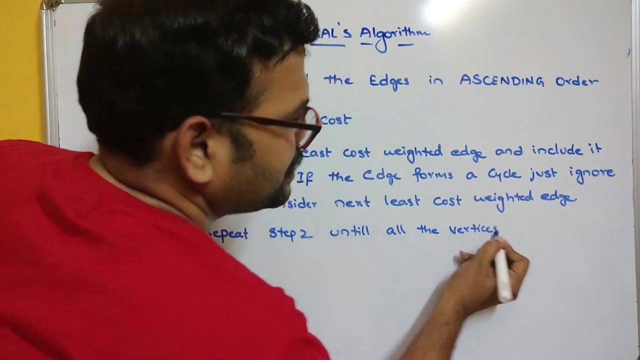 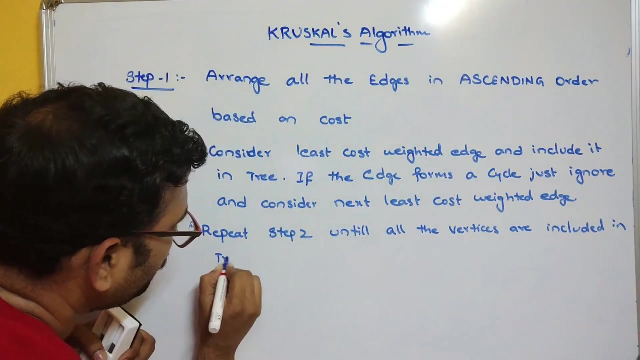 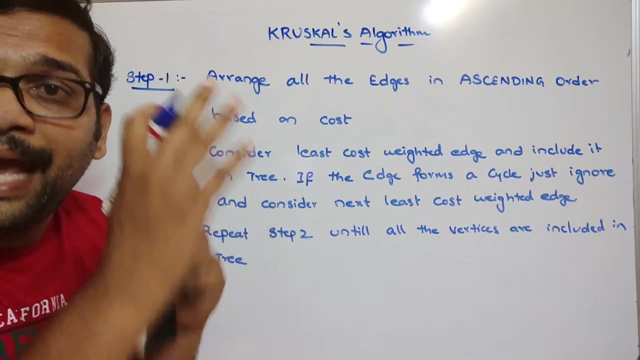 And the third step. third step, repeat step two until all the vertices. all the vertices are included in a tree, included in tree. So we know the spanning tree right. So if the tree is having, if the graph is having some n vertices, then the spanning tree should have the n vertices. 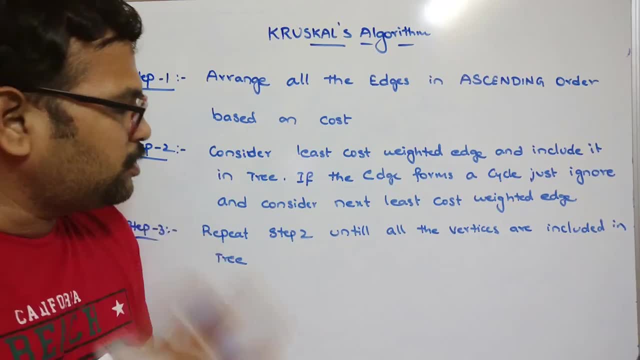 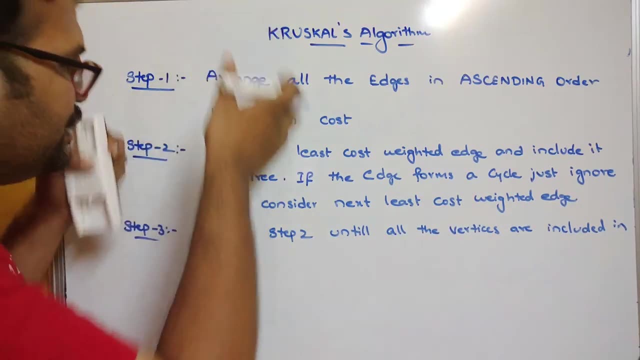 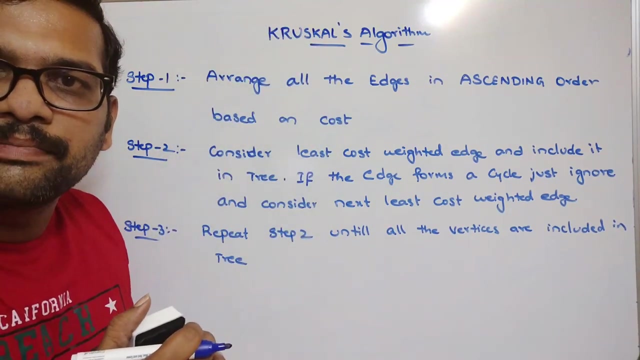 with n minus one edges right. So similarly we have to repeat the step two until all the vertices are included in a tree. So by following these steps we can find the minimum cost spanning tree by using this Kruskal's algorithm. 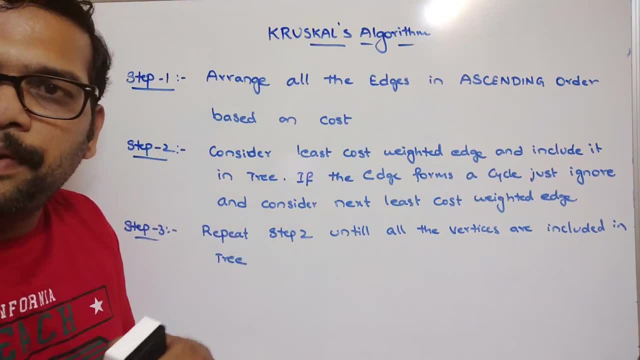 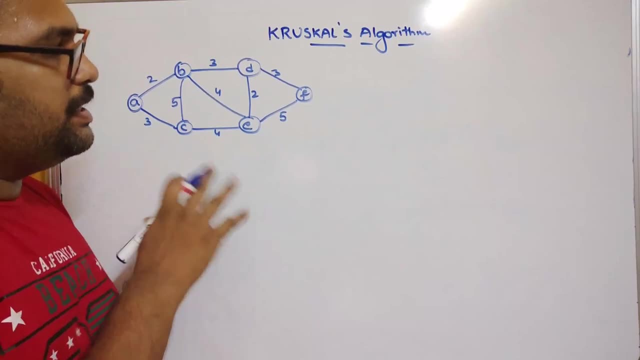 Right, So hope you understood this one. and now we'll see an example and we'll find the minimum cost spanning tree. So let us consider this example, And this is a graph, and we need to find the minimum cost worth spanning tree. So what's the first step? 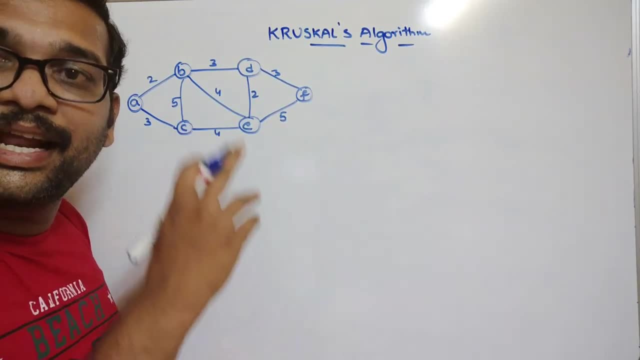 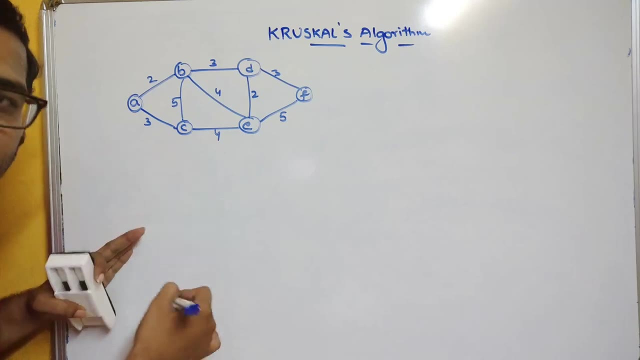 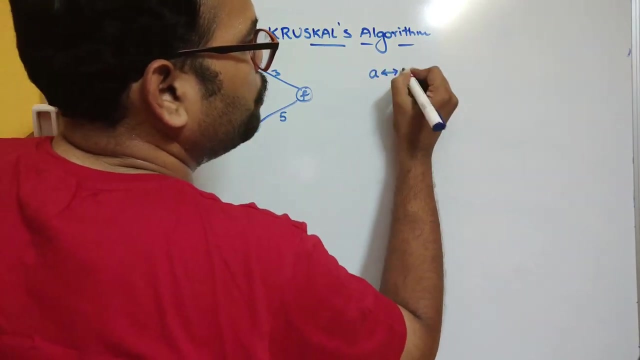 We have to arrange all the edges in an ascending order based upon their cost. So here the first. the cost among these things are 2. so first let me write all the edges with a 2. so here you can see A to B. A to B is a 2 with a cost 2. so this is a bi-directional. 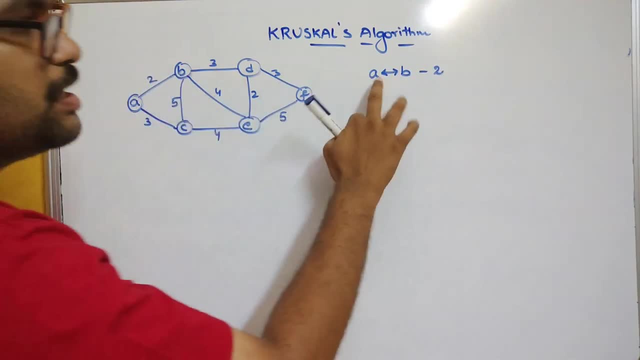 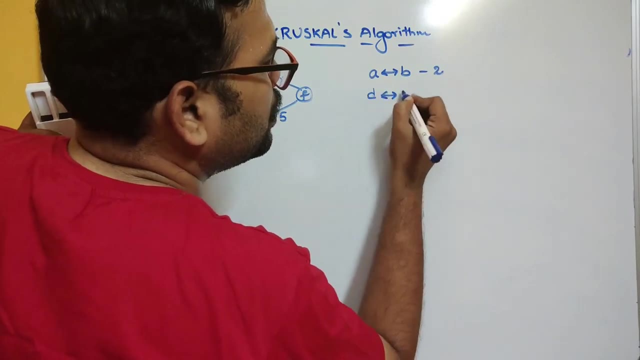 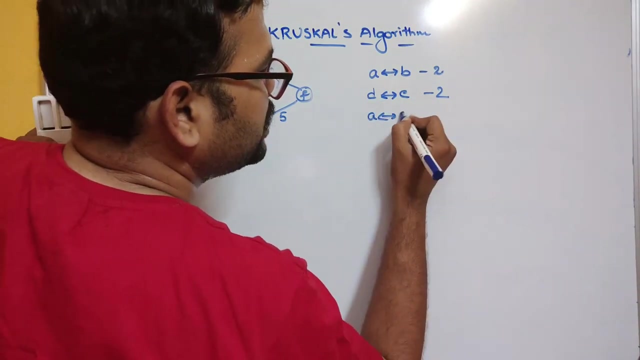 because this is this is a bi-directional. we can simply consider A to B or B to A. next there is a one more thing. there is a 2, D to E. again it is a 2, next 3. so we are having A to C, A to C with a, 3 and one more: B to D with 2, d with a. 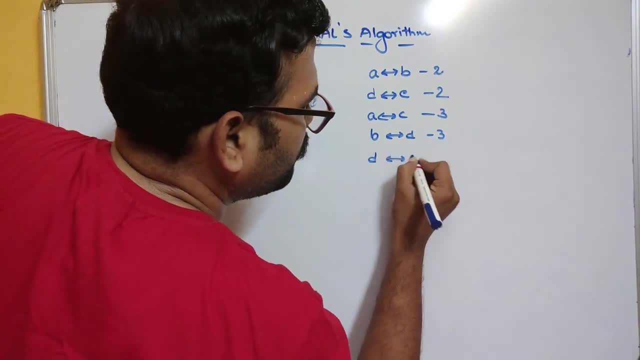 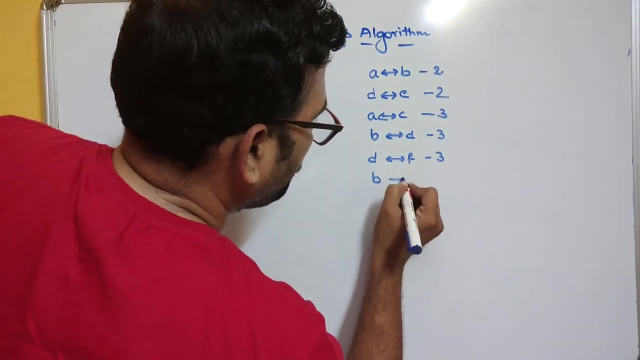 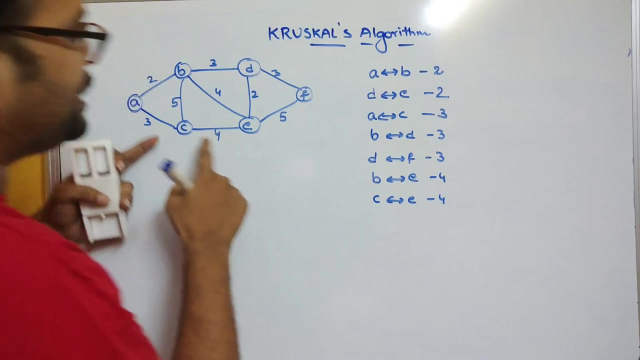 cost 3, and D to F, d2f with a cost 3. then what about? next one is the 4, so 4. B to D, B to E with a 4 and C to E with a 4. next one is 5, so B to C. 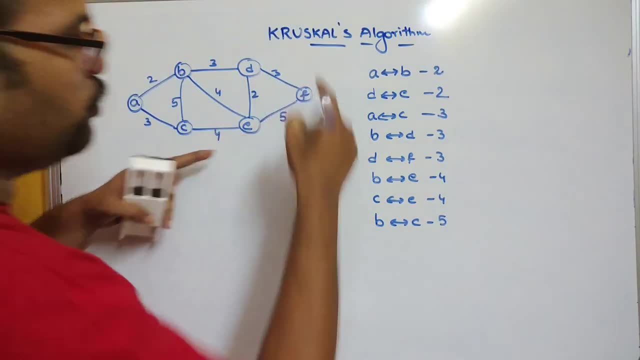 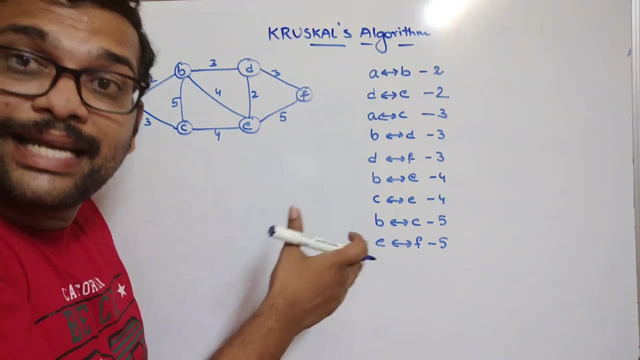 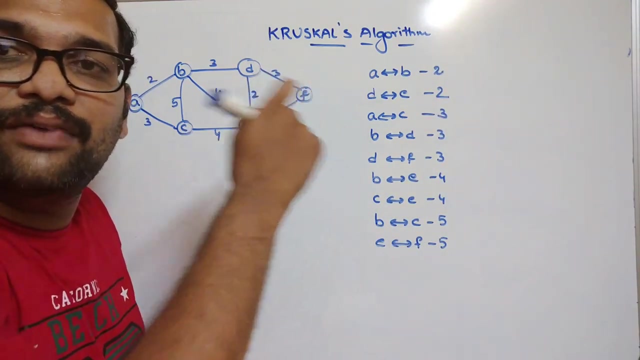 5, and E to F is 5.. So you can observe. these are the edges arranged in ascending order, because you can observe the cost. So from lower to higher. Now what is the first step? Consider each and every least costed edge and include it in tree. So first consider, 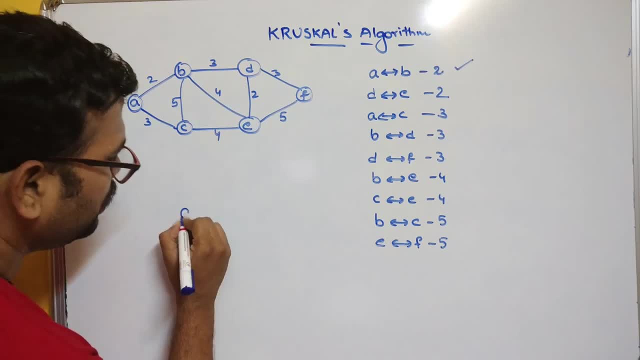 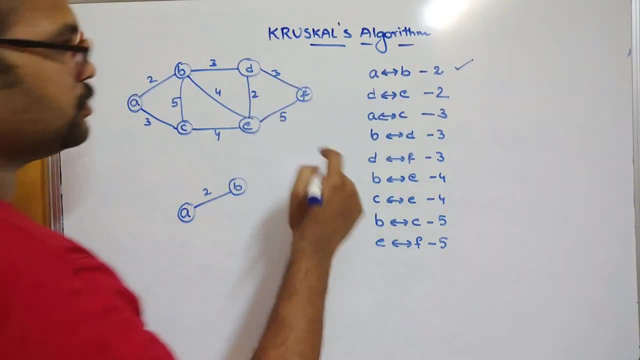 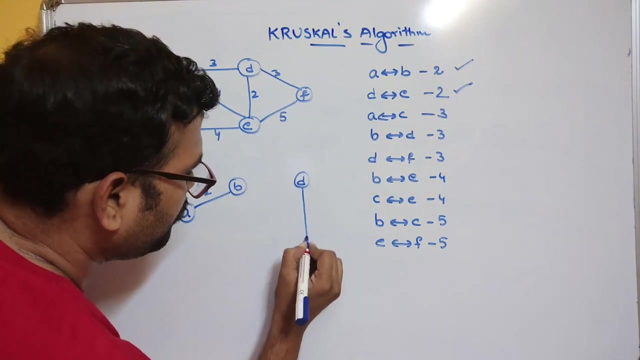 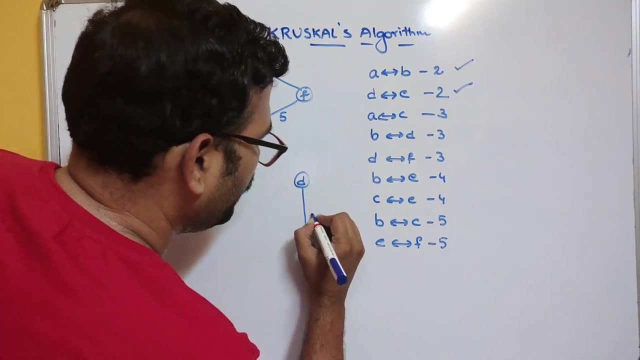 A to B. So I will construct the tree here. So A, B, which will cost 2.. Next step: D to E, So D to E, So D to E. So here it is a, D, E. So what is this one? D to E again. 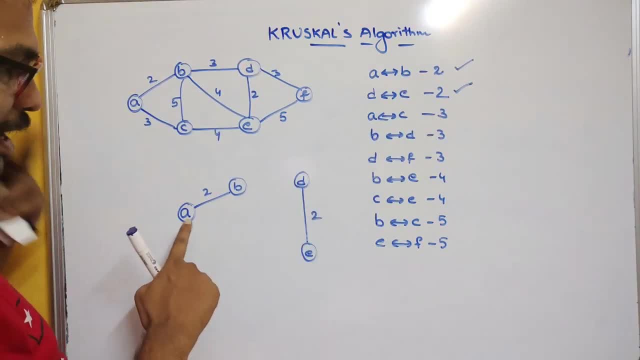 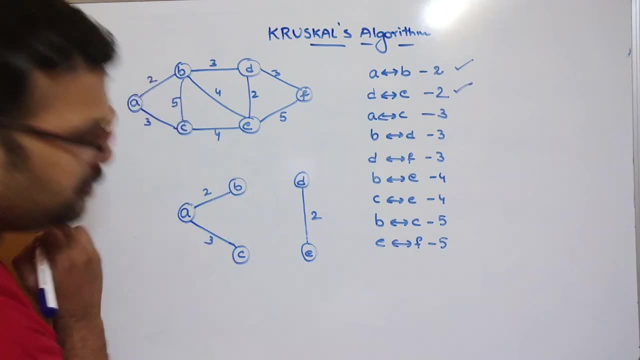 2. Next A to C. 3. A to C. there is no C, So we have to add it A to C. 3. Next B to D. B to D, So it does not form the cycle. 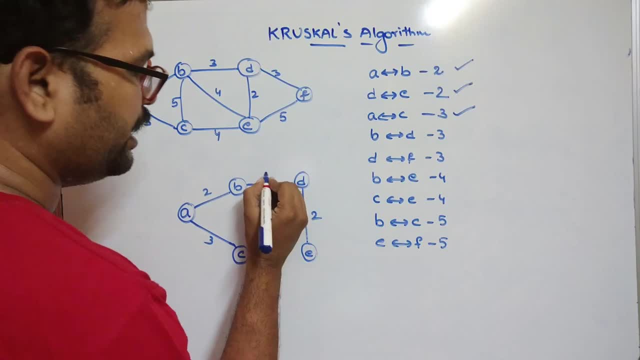 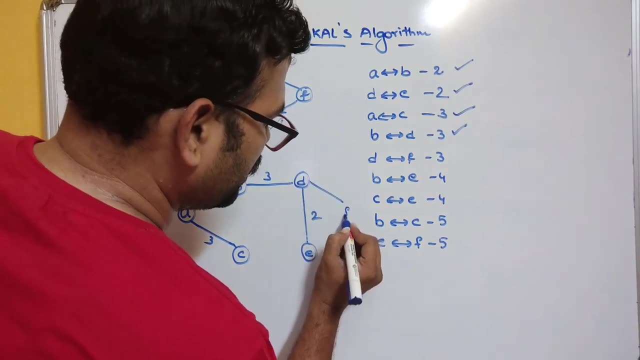 right B to D. So just include that one B to D, again, it is 3.. Next D to F. So there is no cycle. So I will construct here F. D to F, it is 3, right. Next B to E. So 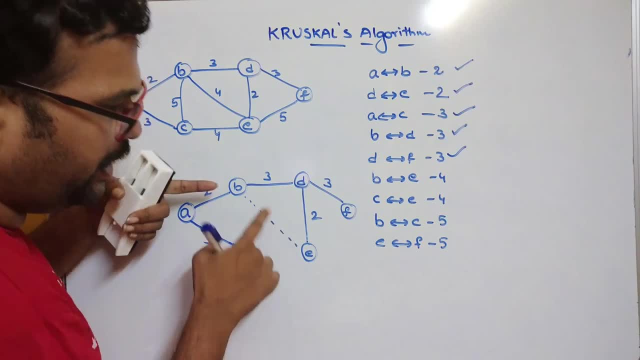 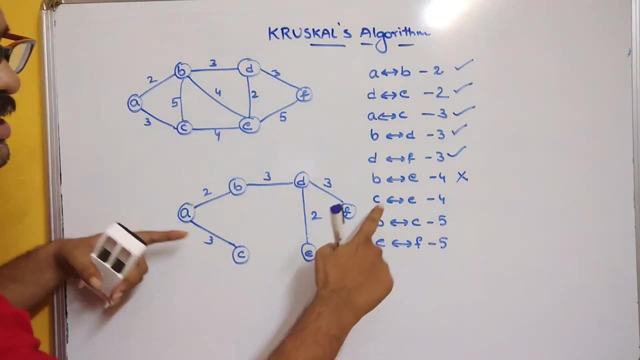 if you, if you give the edge here, B to E, it forms a cycle. right, It forms a cycle. So we should not consider this one. So this should be rejected. C to E, C to E. Again, if you form an edge. 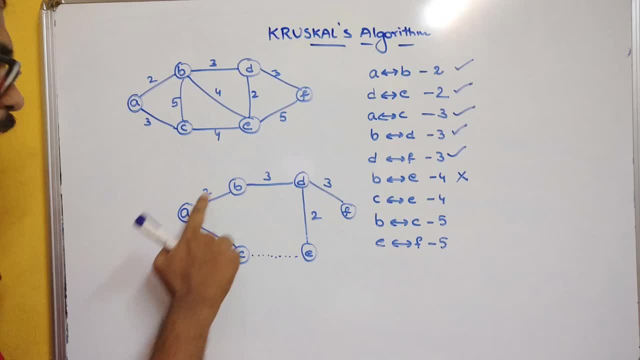 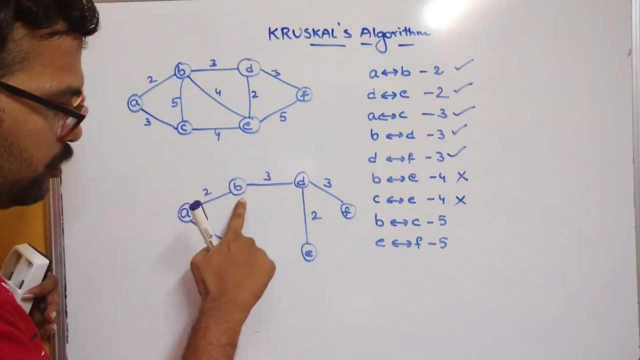 if you give an edge again it forms a cycle- right A, B, D, E, C, A. So we have to reject that. B to C, B to C Again. if you form an edge, so it forms a cycle. So we have to. 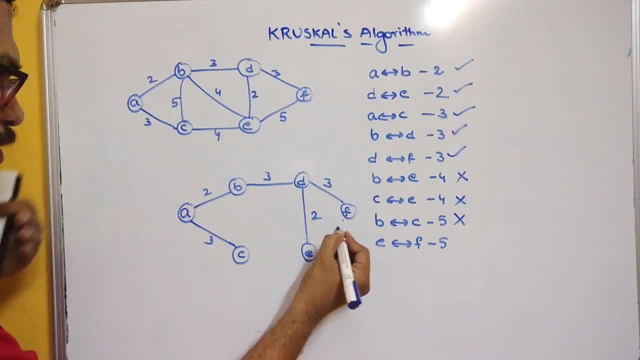 reject: E to F, E to F. If you consider the edge here again it forms a cycle. So you have to reject. So you can see in our graph there are 6 vertices, 6 vertices and our. 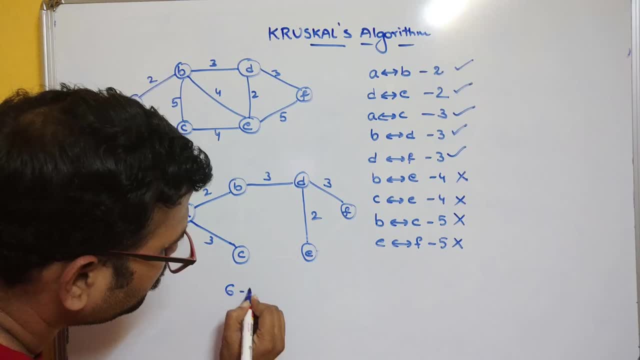 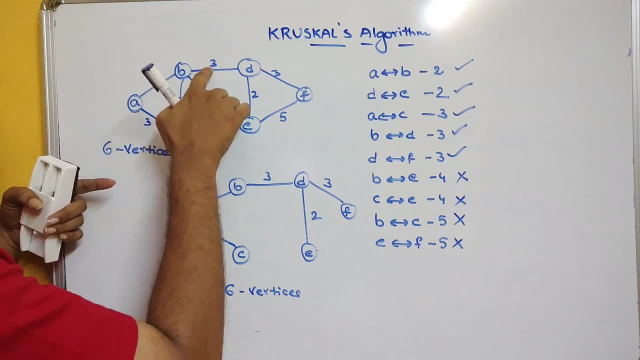 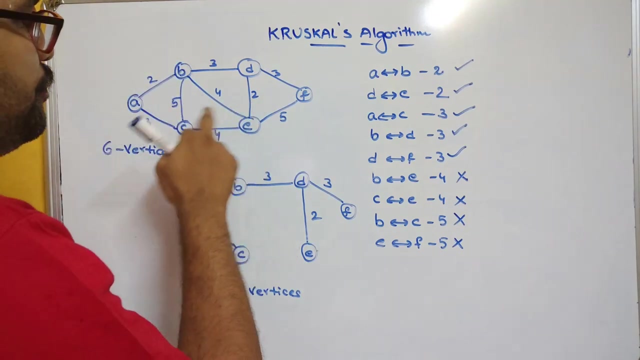 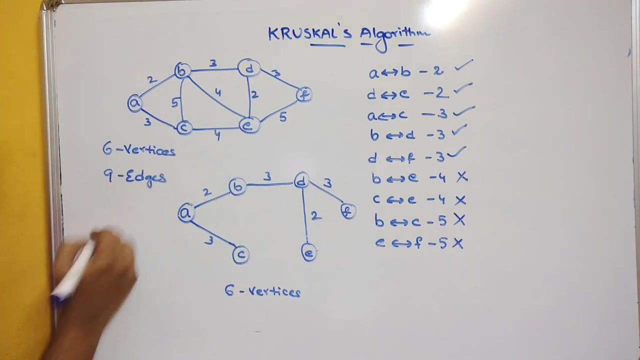 spanning tree consists of 6 vertices, 6 vertices right And here the edges 1,, 2,, 3,, 4,, 5,, 6,, 7,, 8, and 9.. Okay, So 3,, 6,, 7,, 8,, 9 edges. So there are 9 edges You can observe here: 1,, 2,, 3,, 4,. 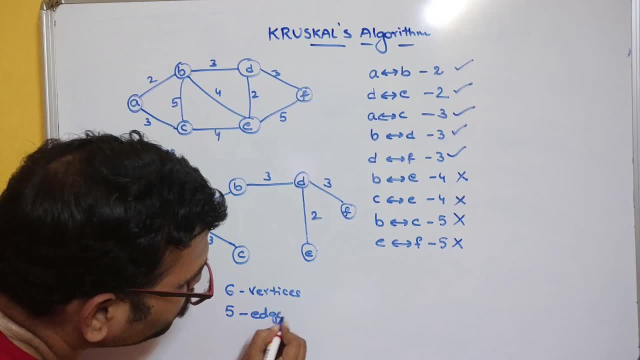 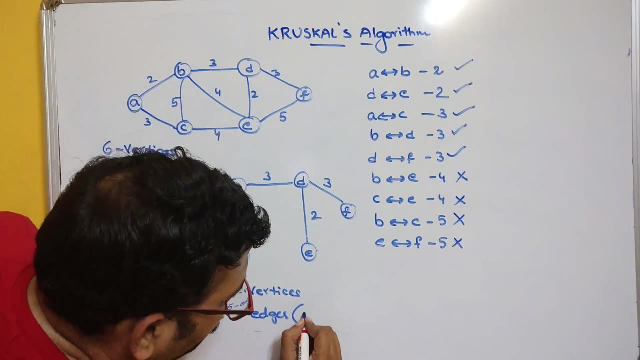 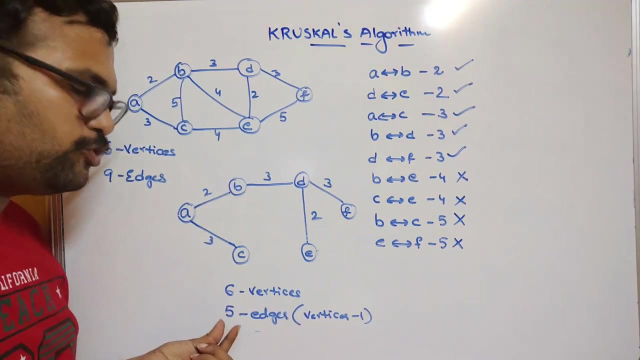 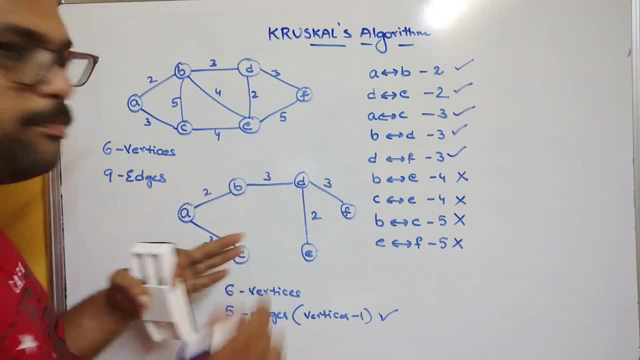 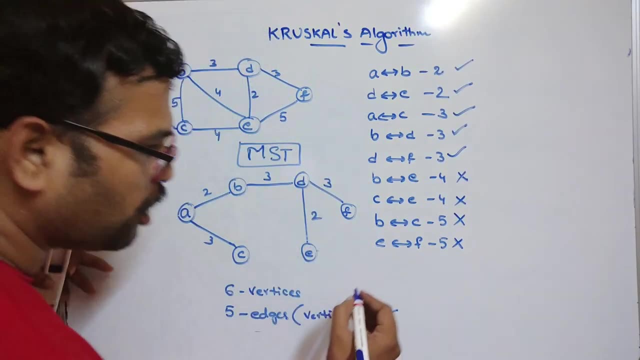 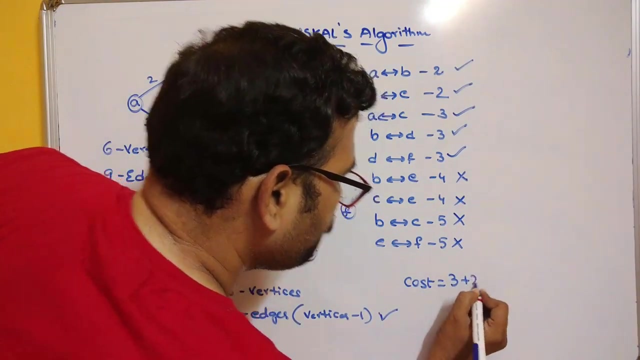 covered. So we can consider this as a minimum cost spanning tree, which can be represented as MST: minimum cost spanning tree. So now, what is the cost here? Consider cost here. So cost of this one will be 3 plus 2 plus 3 plus 3 plus 2.. 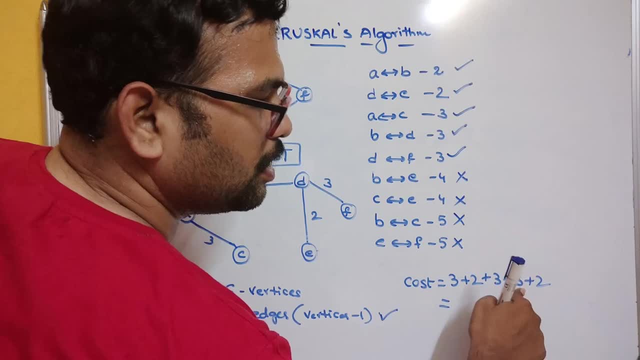 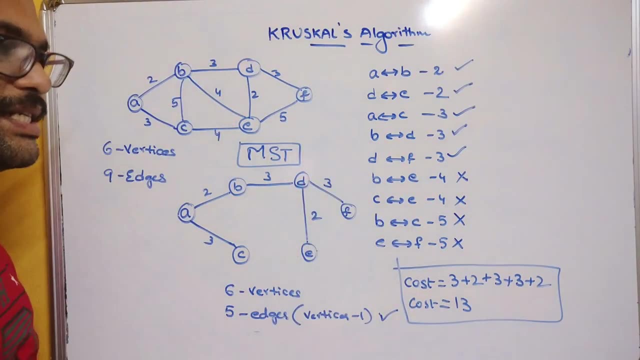 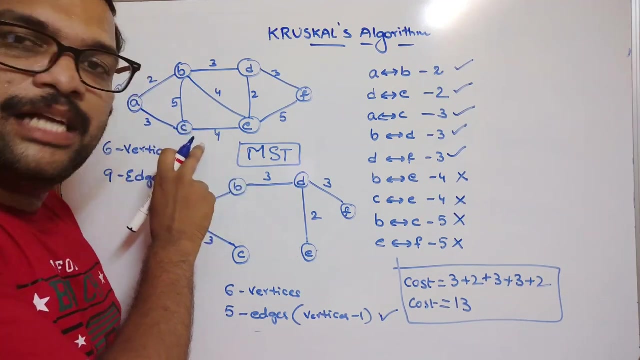 So the cost will be 5,, 8,, 11, and 13.. So cost is 13.. So the minimum cost we can create or construct the spanning tree is with 13.. So you just remember. this is the same example. 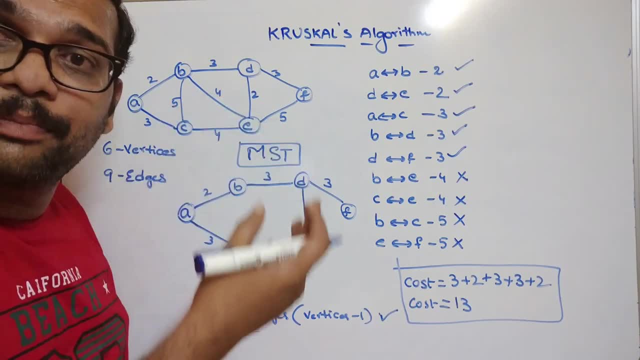 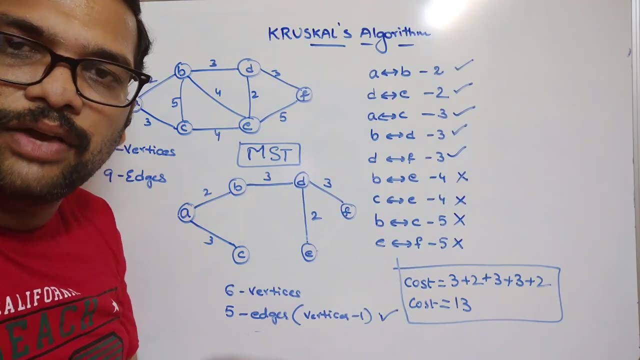 we have taken in the PRIMS algorithm also. So there also we have constructed the minimum cost spanning tree with a cost of 13.. So once just observe the session. So I will post the link in the description So you can follow that one. So that is the procedure of PRIMS and this is the procedure. 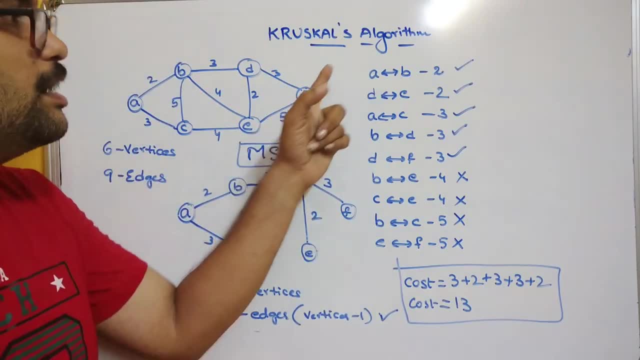 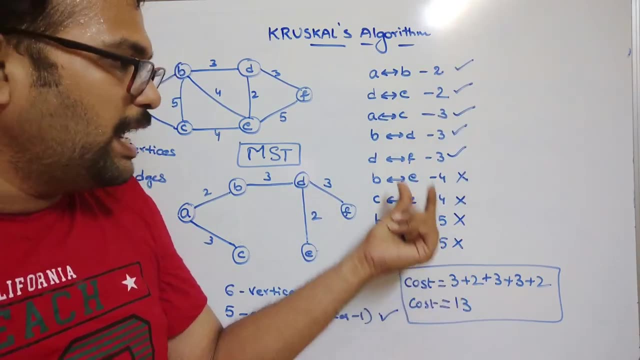 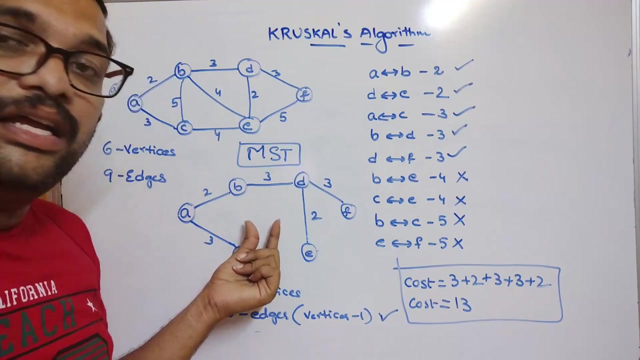 we need to follow for the Kruskal's. So this procedure is Kruskal's algorithm. So first we have to arrange all the edges in an ascending order based upon their cost and then consider each and every edge and construct a tree. And if, by adding the edge to the tree, if, 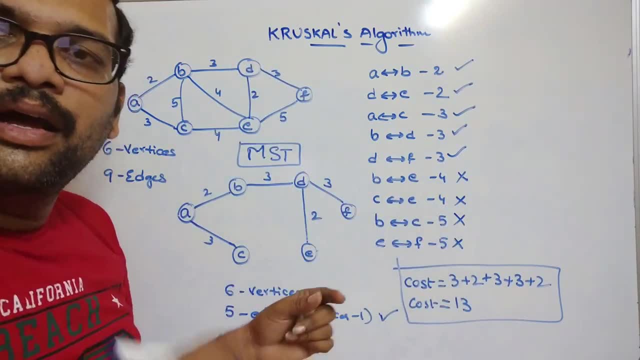 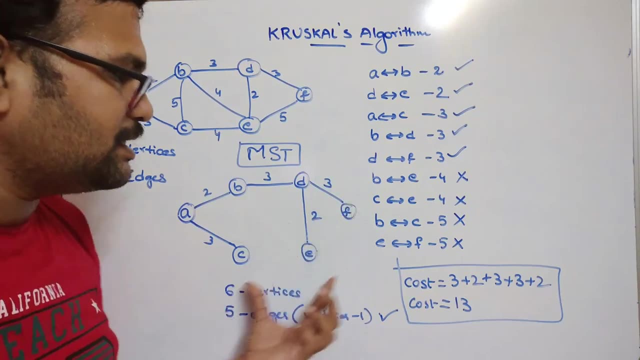 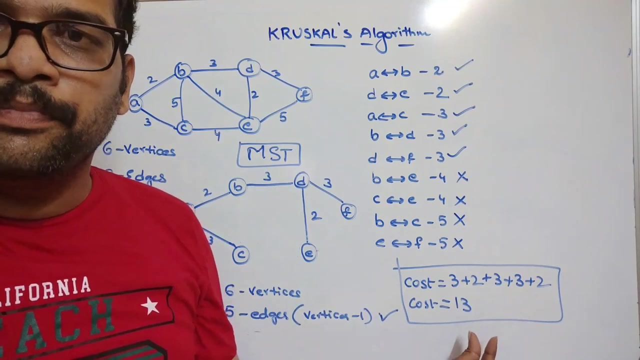 it forms a cycle. just ignore that and consider the next least cost edge, Right? So we have to repeat that one until all the vertices are covered. So here there are 6 vertices. All the 6 vertices have been covered with a cost of 13. Right, So hope you understood. 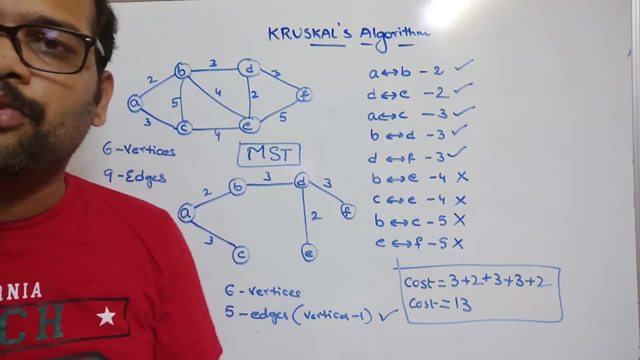 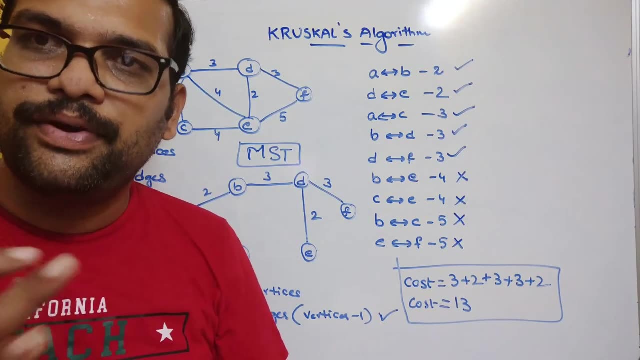 this one. So this is a Kruskal's algorithm to find the minimum cost spanning tree Right. So if you are having any doubts regarding this one, feel free to post your doubts in the comment section. Definitely, I will try to clarify all your doubts And if you really 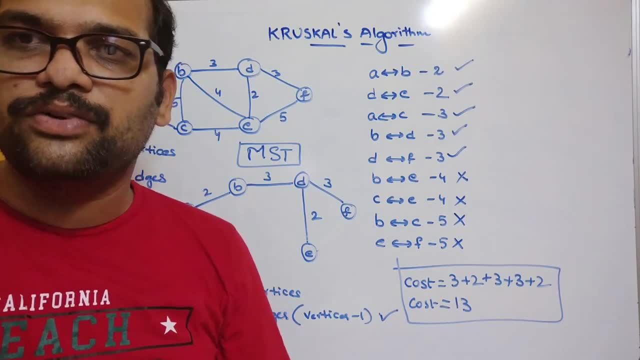 enjoyed my session. like my session. share my session with your friends and don't forget to subscribe to our channel. Thanks for watching. Thank you very much.